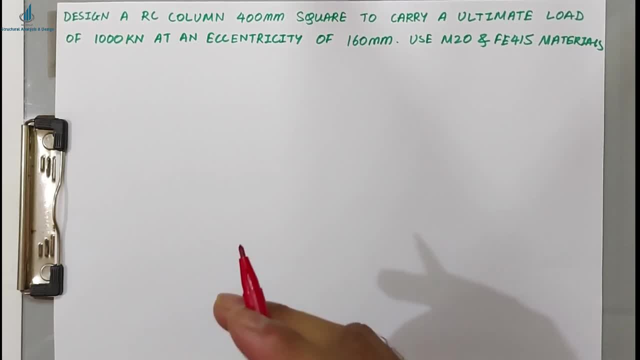 sense, as per the IS code, we had to provide 20 mm eccentricity and we have solved square, rectangle and circular column based on that minimum eccentricity concept or axially loaded concept. So in this video we will see a RC column which is a square and it carries 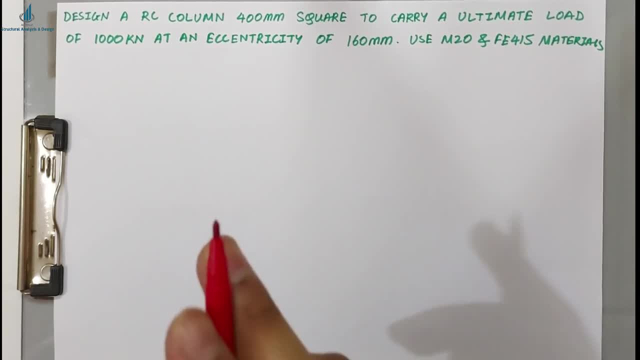 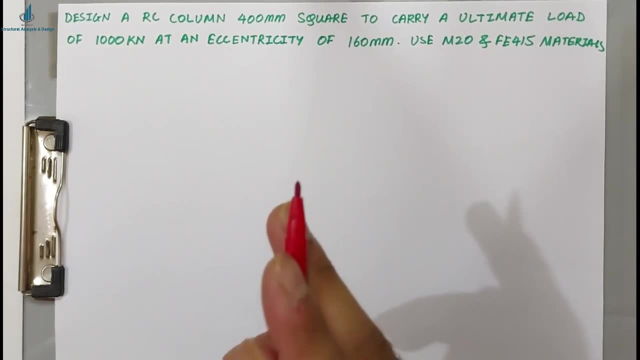 a axial load but it also has an eccentricity, So it is a column with axial load and uniaxial bending. So I will be sharing the link in the description box of my previous column videos So you can just check out those videos. 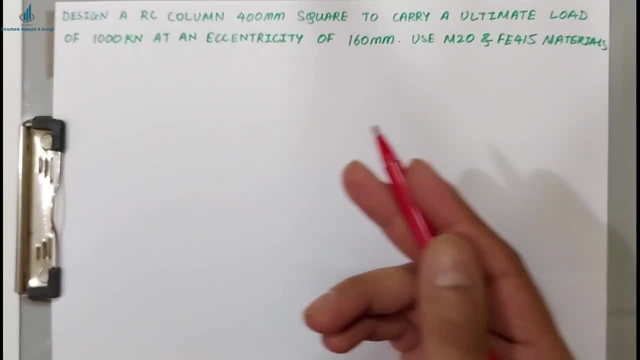 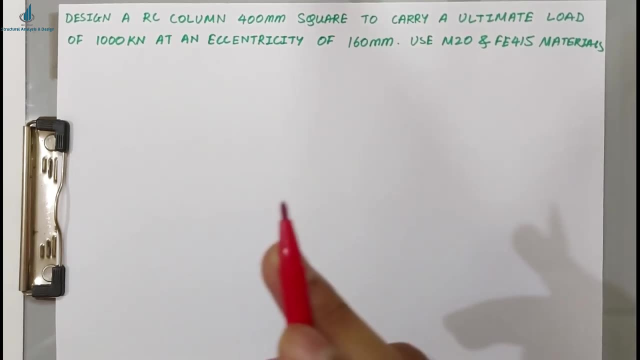 videos and you can further study this particular uniaxial bending column. So let's start with this today's video And if you want to have a knowledge about what is uniaxial bending and biaxial bending, that also link I will be sharing in the description box and also on top iCard button. 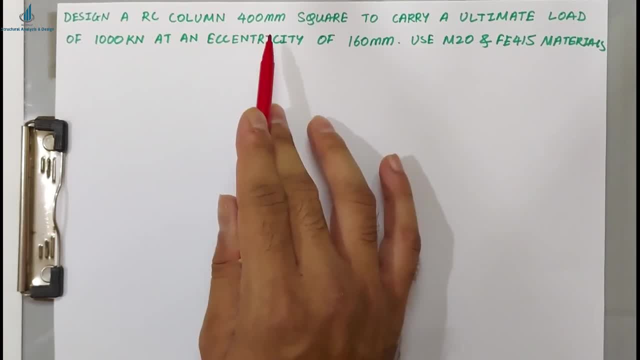 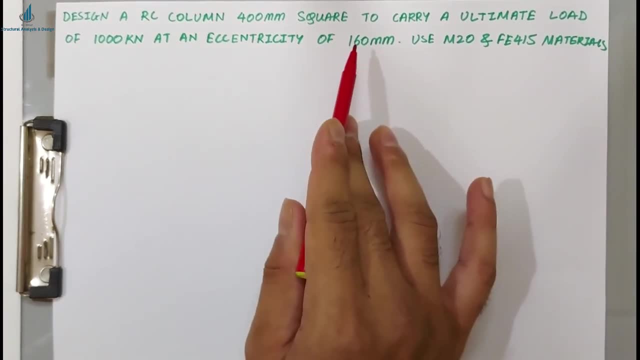 In this today's problem. they have given design a RC column, 400 mm square, to carry a ultimate load of 1000 kilo Newton at an eccentricity of 160 mm. So if you see the word eccentricity then you need to have a knowledge of uniaxial bending. 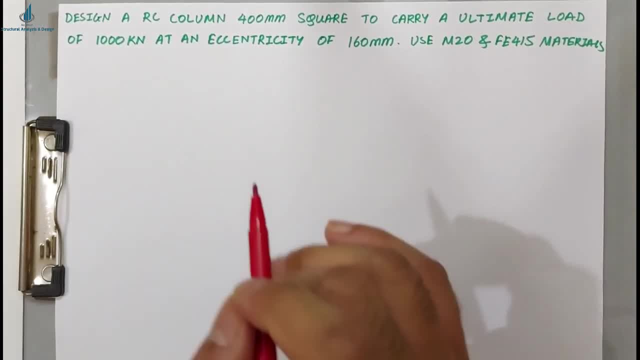 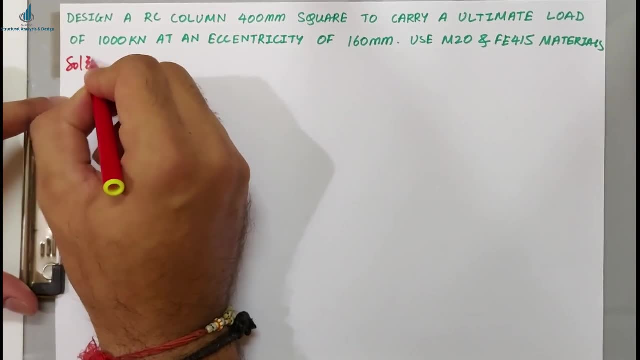 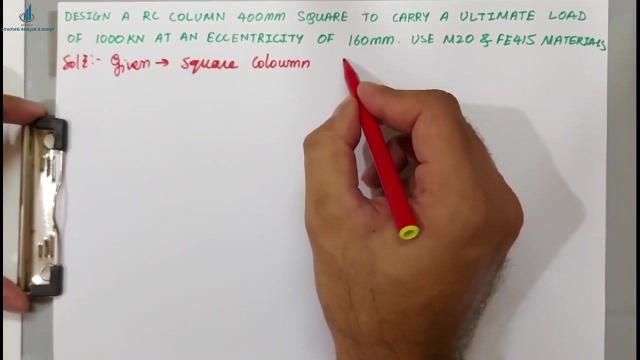 and you have to use M20 and FE415 materials. So first, as a usual practice in RCC design, you will write down the given data. So solution given. So the column type is square column. Then B, Okay, Equals to D, equals to 400 mm. 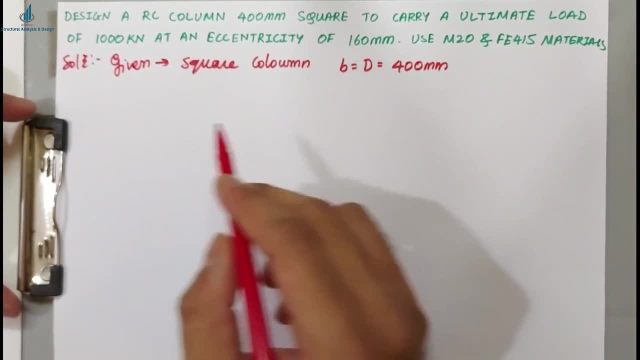 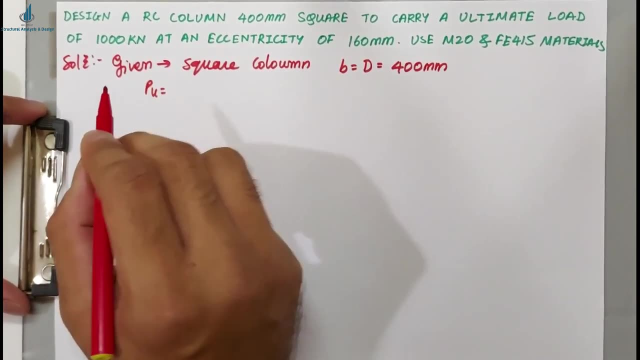 B is equals to D because it is a square column. And next thing, they have given ultimate load. Okay, So directly PU. they have given not only load, they have given ultimate load. no need to multiply by 1.5. factor of safety. 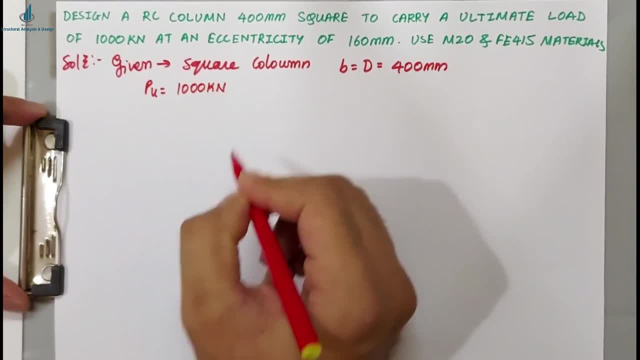 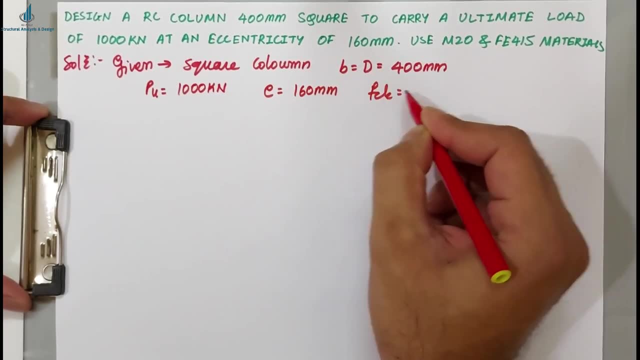 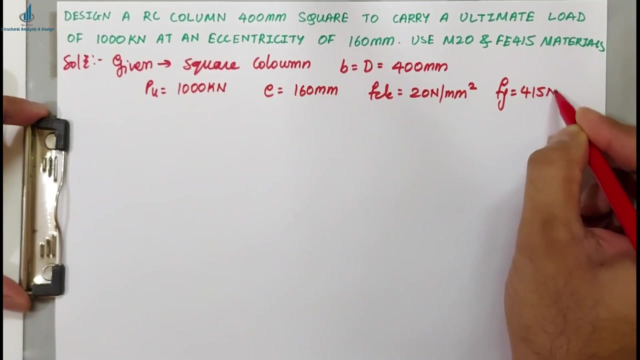 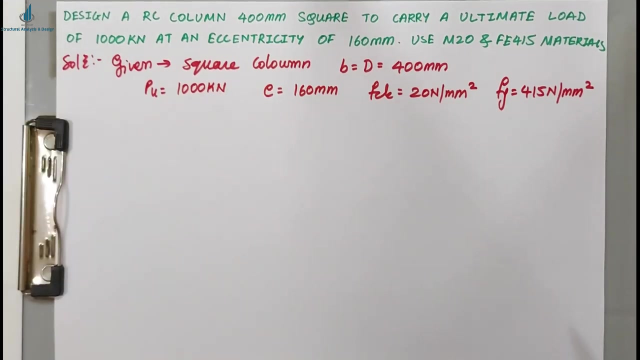 So directly you can use this 1000 kilo Newton. Then eccentricity, they have given 160 mm And concrete grade, FCK, 20 Newton per mm square And FY415 Newton per mm square. So before proceeding to this problem, the special publication 16 that is also known. 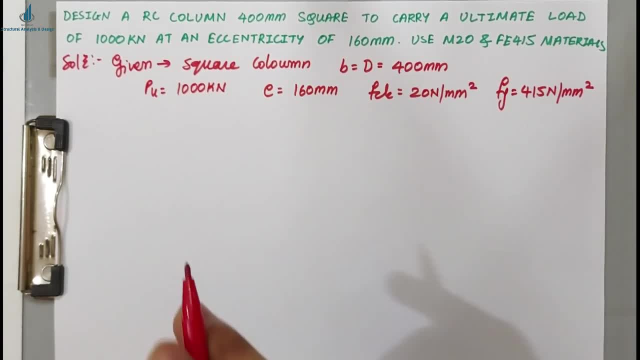 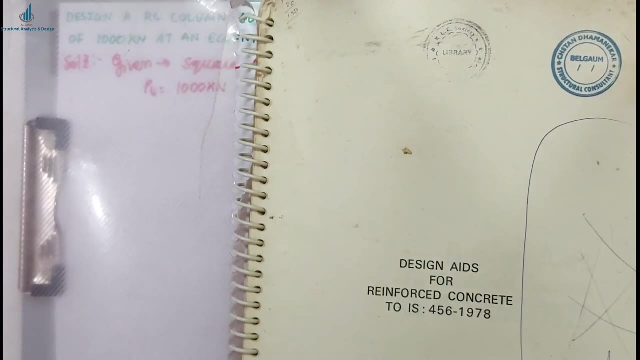 as SP 16, which is a special aid for IS 456 2000.. So I will, I would like to show this SP 16. before proceeding to this problem. So this is the design aid for reinforced concrete IS456-1978. 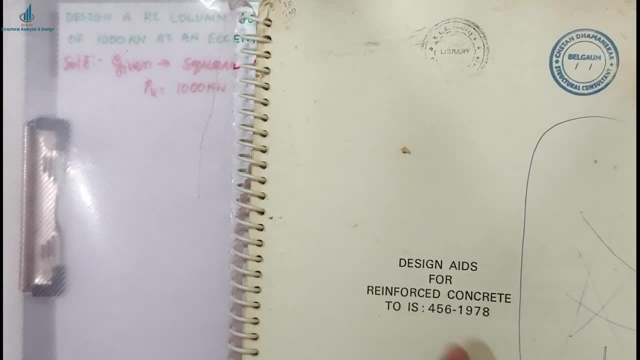 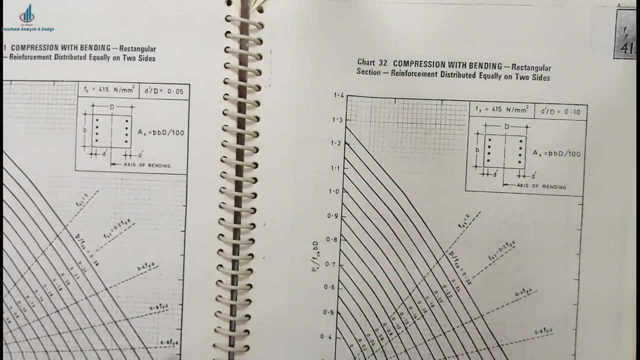 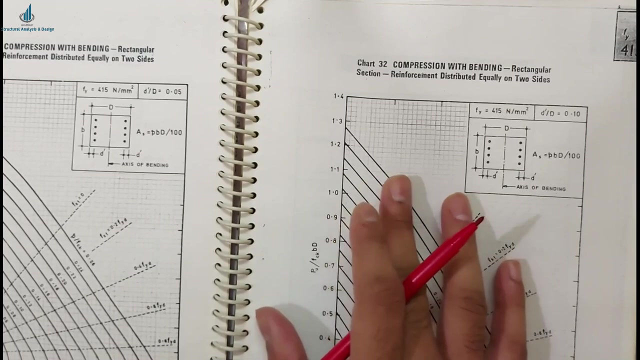 still upgrade. they have not done for 2000 IS456-2000, so same code you can use it. So here it is very simple to solve this type of uniaxial problems. So these type of charts you will be getting in SP16 publication, that is special publication 16, which is design aid for IS456-2000. 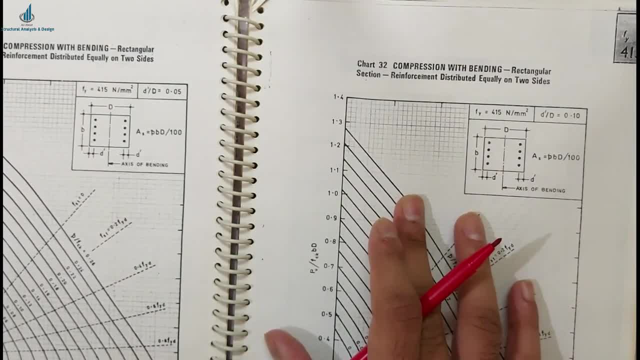 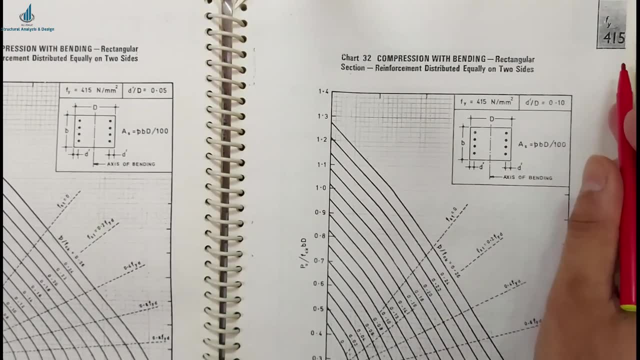 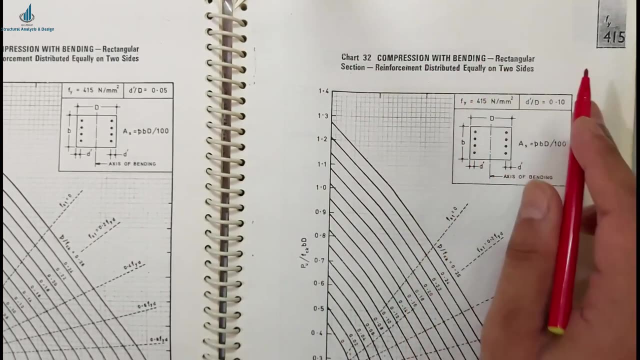 so these are the charts. you will be getting different charts to solve a column with uniaxial bending. So whatever chart I am showing here, it is for grade FY415, so the steel which we are using is 415 and this chart, number 32, we will be using. So before that, I would like to show you this. 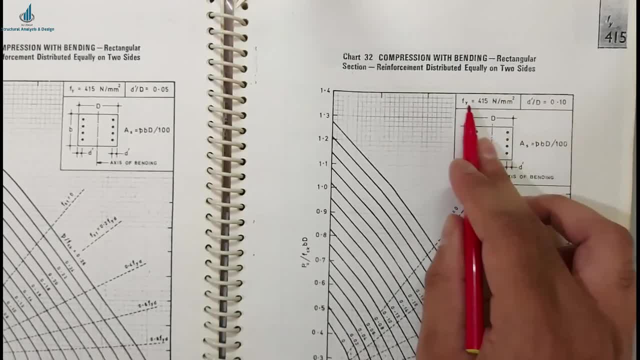 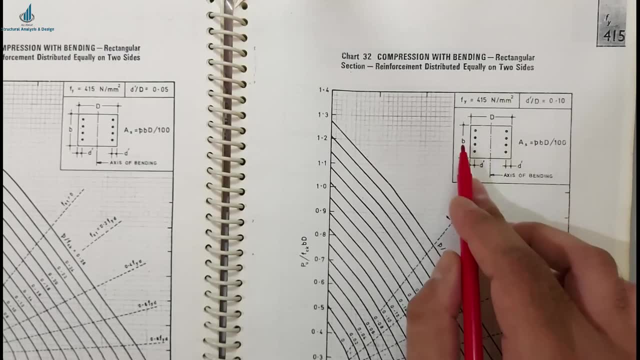 small box here. There is a small box here, So before that I would like to show you this small box. Here they are mentioned: the grade of steel, then D' by D ratio and the arrangement of column reinforcement. So clearly they have mentioned reinforcement distributed equally on two sides and, if you 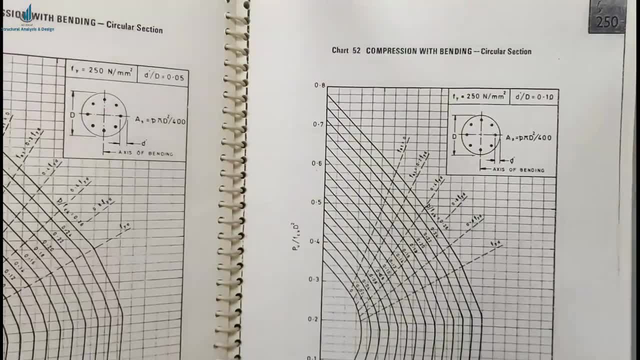 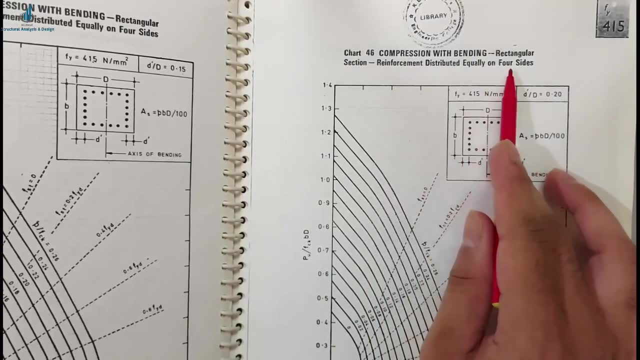 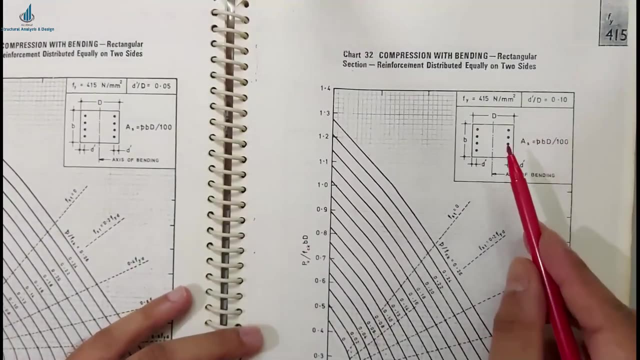 further go into this SP16 publication, you will be having these type of charts where they show reinforcement distributed equally on all four sides. So either you can provide the reinforcement all the four sides or you can provide only on two sides. So this problem which I will be showing, 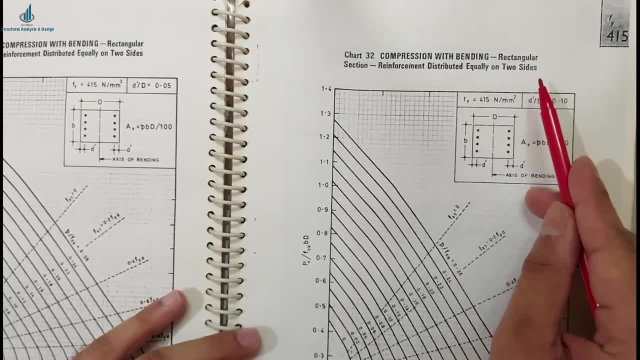 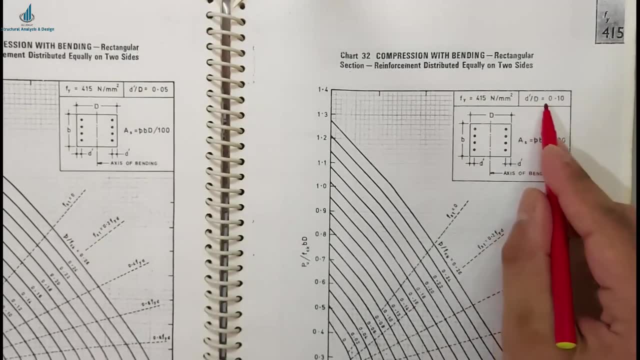 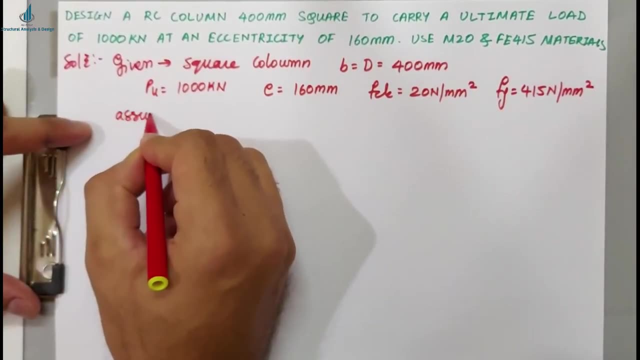 is with reinforcement distributed equally on two sides. So it is very important to have SP16. before moving on to this problem, You require here D' by D, So you have to assume first the cover of concrete. So assume D' equals to 40 mm. Therefore, 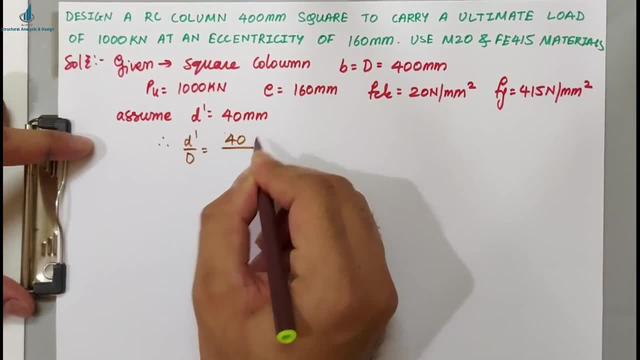 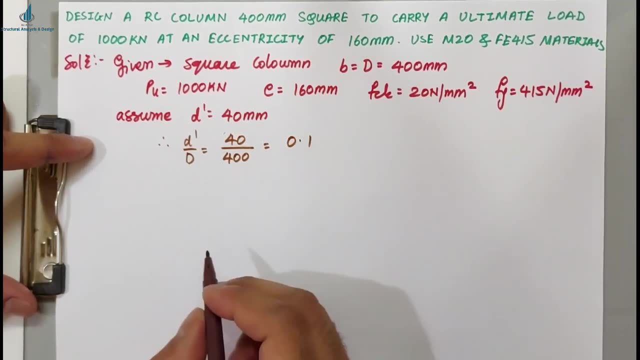 D' by D. So D' is 40 and D is 400.. So you will be getting: D' by D is 0.1.. Now MU, you have to calculate because this eccentricity will create a moment. So MU is equals to PU into E, So PU is 1000 kilo Newton. 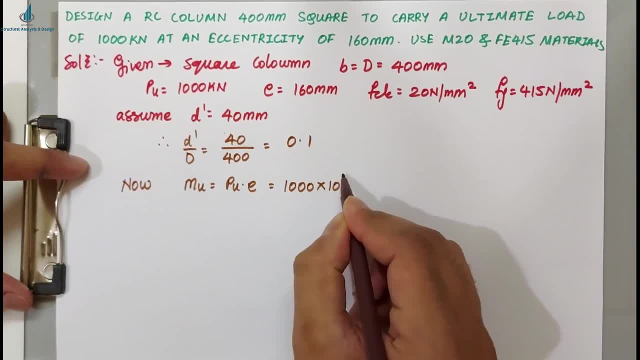 So is equal to the number of millimeters that you took earlier. So we will make a new condition. So I will be converting it into Newtons, because this eccentricity is in mm. So everything we will keep in newton mm. So 1000 into 10, raise to 3 into 160.. So, MU, you will get. 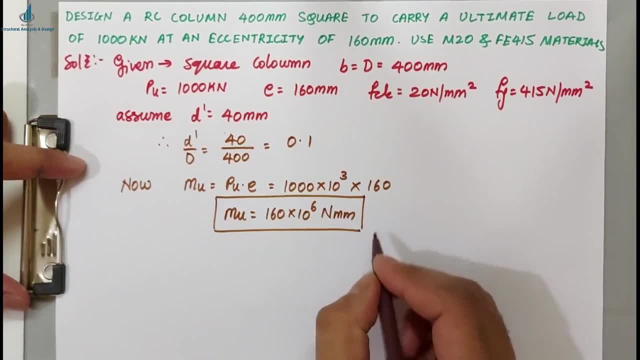 160 into 10, raise to 6 newton millimeter. So this is the next step Now. So M is equal to 0.1 and M is equal to 0.1, I will write in the Next step Now. 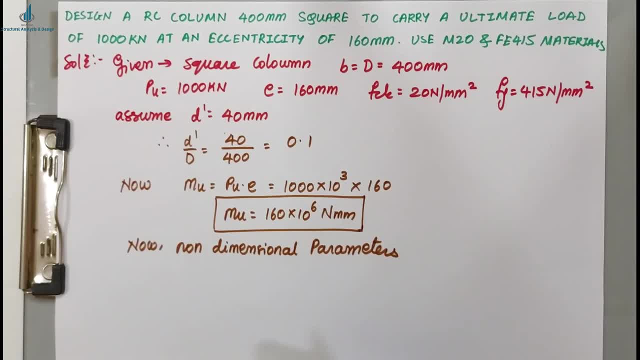 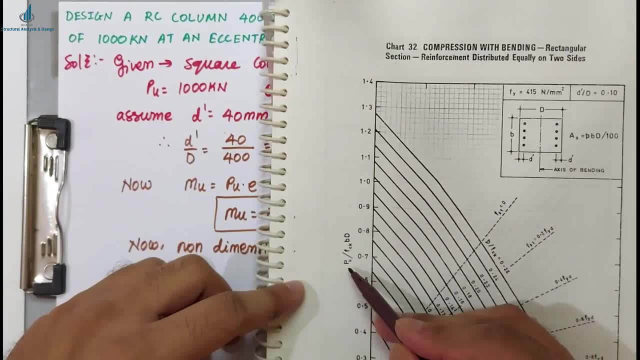 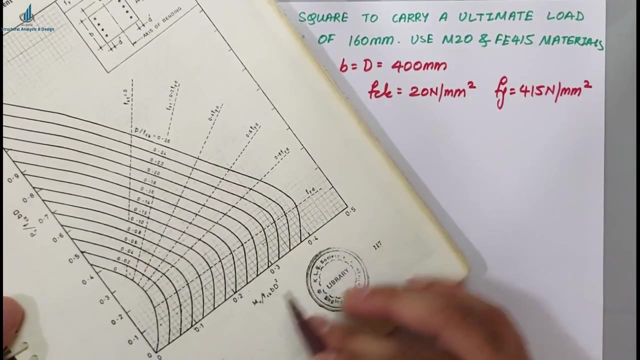 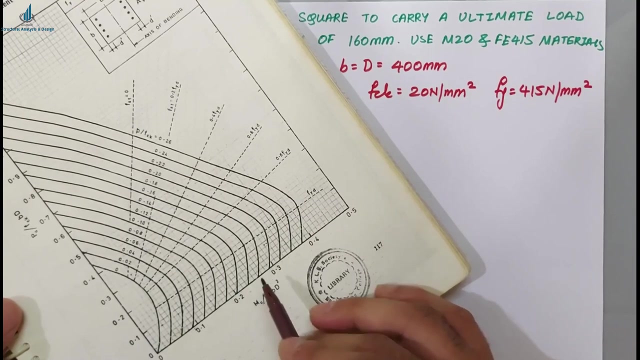 non-dimensional parameters, which is also given in your SP16.. So if you carefully see here, your y-axis is PU by FCK BD and if you see this x-axis it says MU by FCK BD square. So these x-axis and y-axis parameters are known as non-dimensional parameters. So you need to. 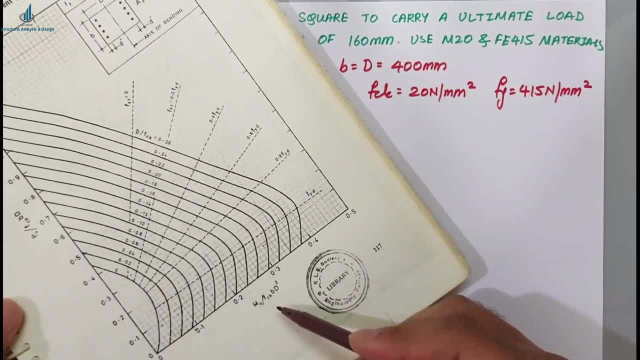 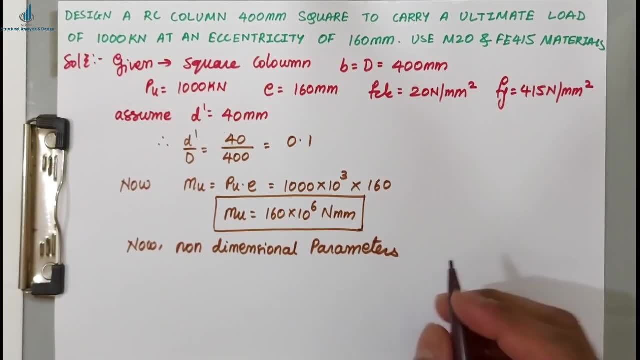 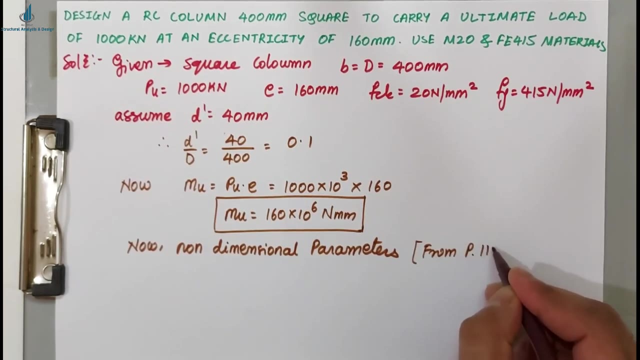 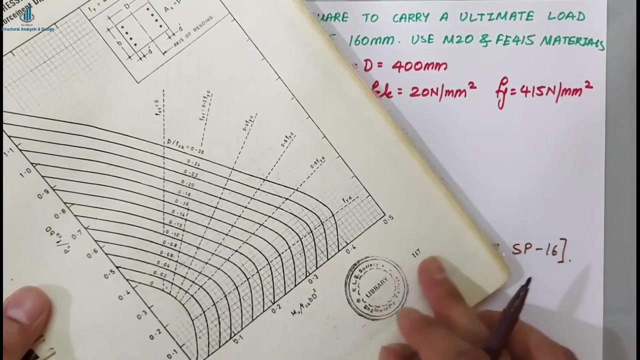 calculate PU by FCK BD and MU by FCK BD square before moving on to this problem, So non-dimensional parameters. So I will write down here from page 117, SP16.. Page number 117 I have mentioned here because we are finding out. 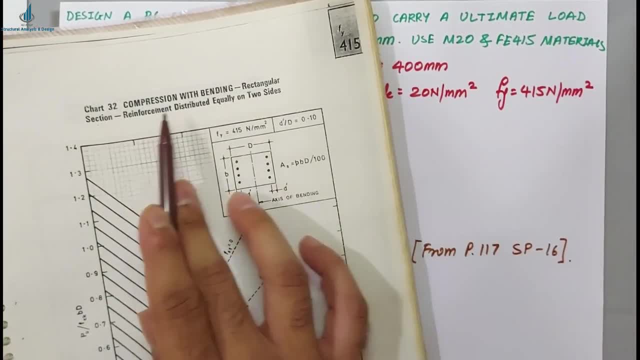 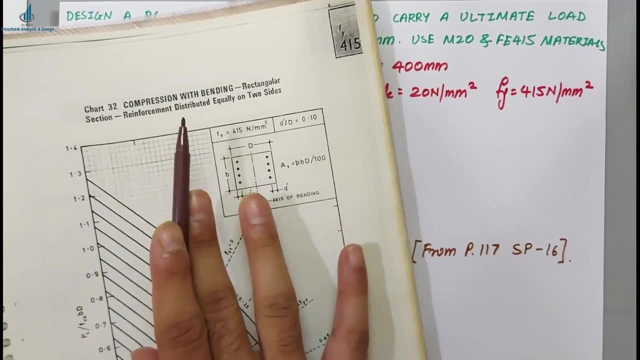 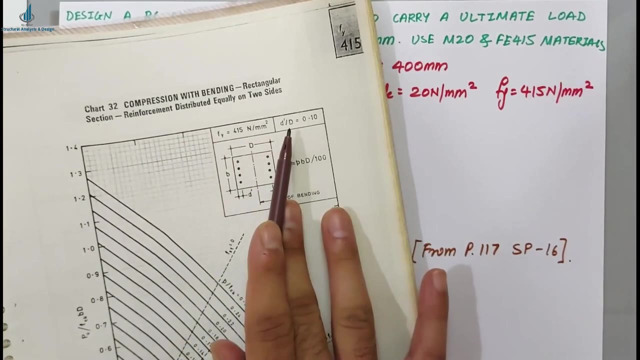 for FY415 material and reinstalling. So the reinforcement distributed is equally on two sides. So this chart, number 32, is applicable for this problem. So, based on your reinforcement distribution and your steel grade and your ratio D, dash by D, other charts also you may use. I will be using these other charts in next. 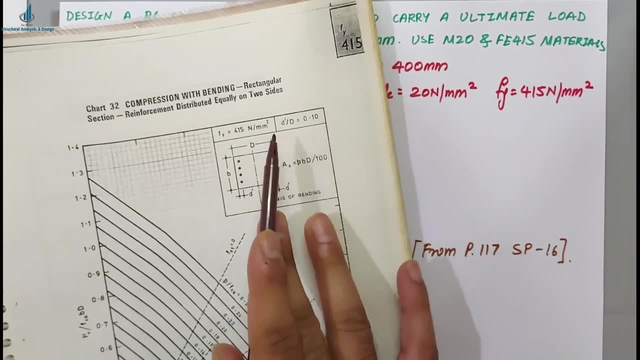 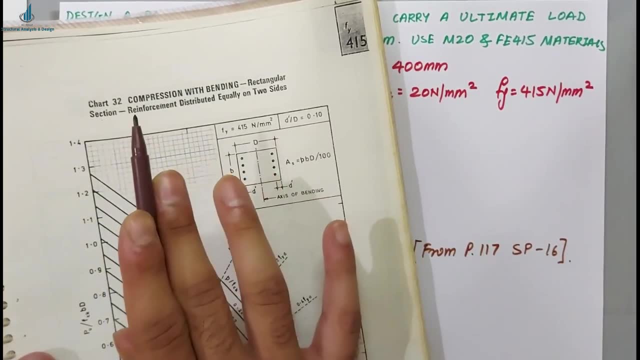 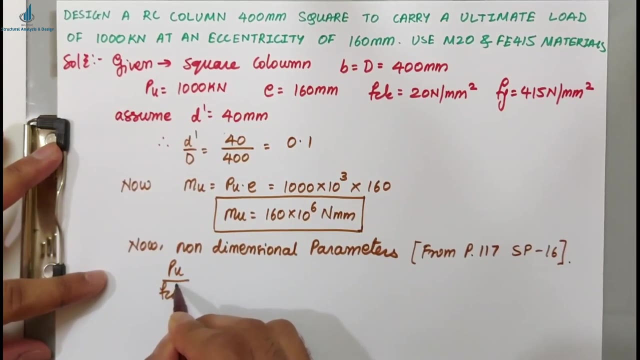 subsequent videos for circular columns as well as rectangular column also. So for now we will be using this chart, number 32 of IS sorry, of sp 16. so the first is pu by fck bd. so pu is 1000 kilo newton which will be converting it into newton, fck is 20, and b and d are 400. 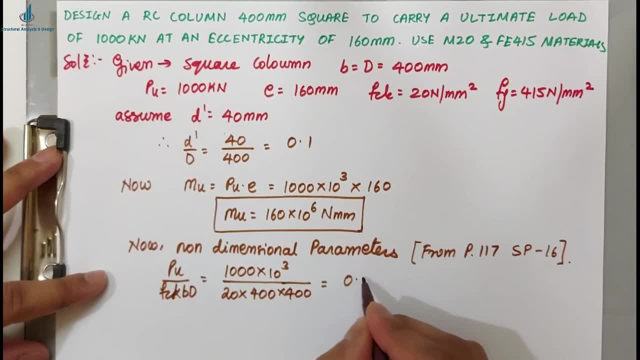 400, so you will be getting this 0.3125. then mu by fck bd square right. so mu is 160 into 10 raised to 6 divided by 20, 400 into 400 square, so you will be getting 0.125 now 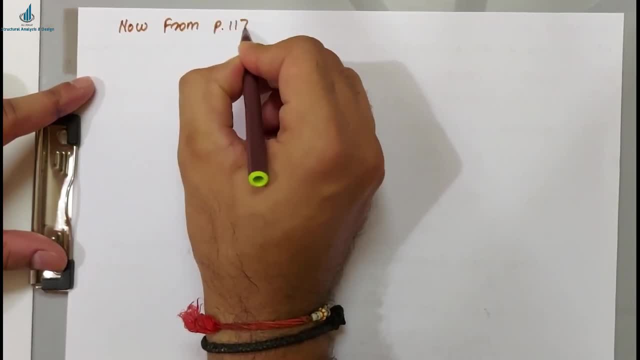 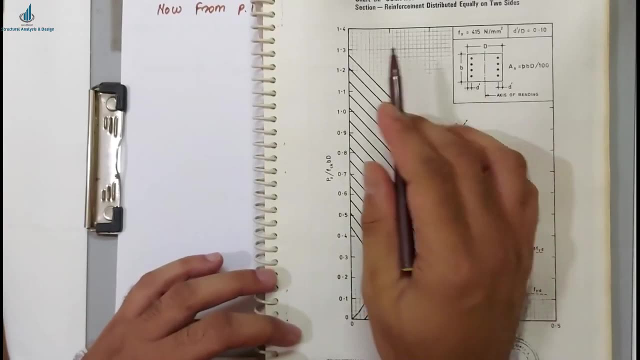 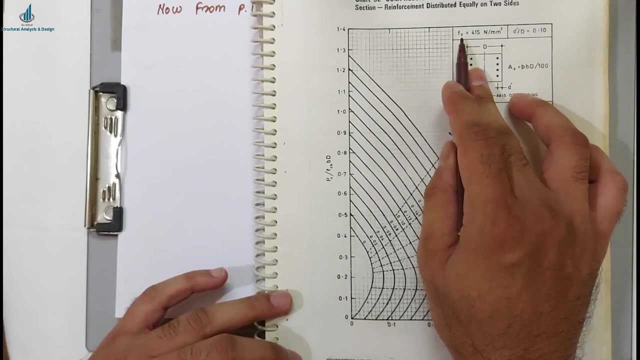 from page 117. chart 32, sp 16. so this is chart number 32, page 117. it is equally on two sides. d dash by d is 0.1 and the grade of steel is 415. so strictly you have to stick with this chart. so now your 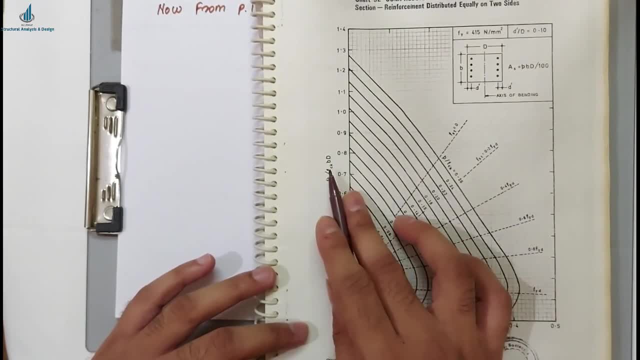 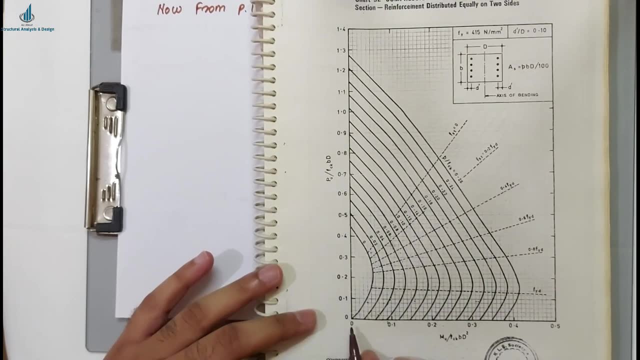 non-dimensional parameters. pu by fck bd was 0.3125. mu by fck bd square was 0.125, so 0.125 means. so the least count of this x-axis is 0.01, so this is 0.1. so this will be 0.11, 0.12 and this will be 0.13. so 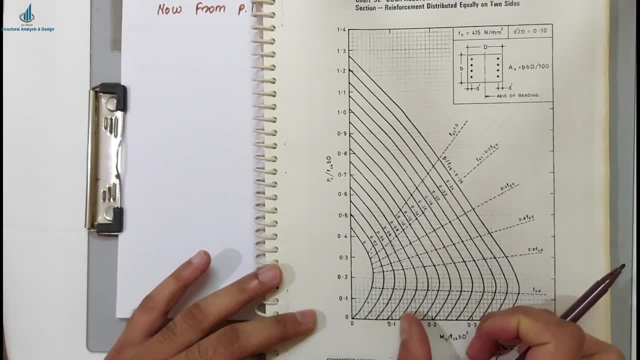 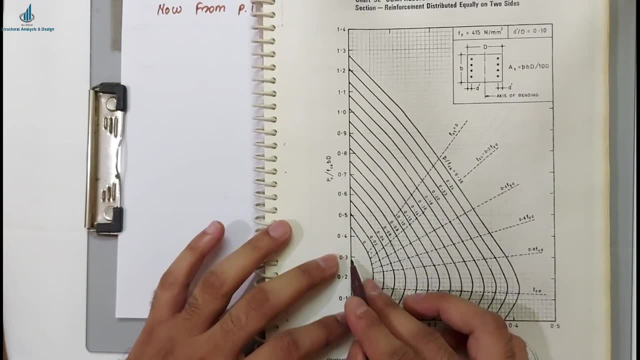 in between. here you will be taking on this x-axis mu by fck bd square and subsequent your pu by fck bd. that is 0.3125. so here the least count is 0.02. so this is 0.3 and the next immediate square will: 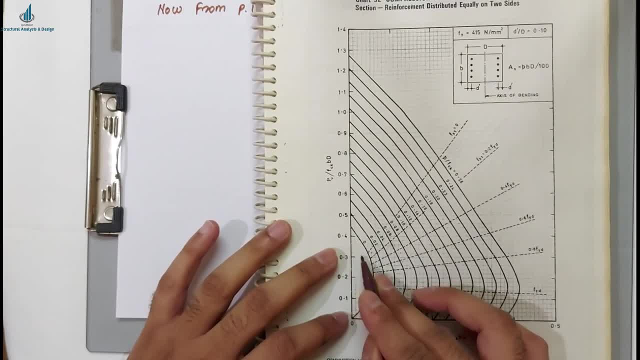 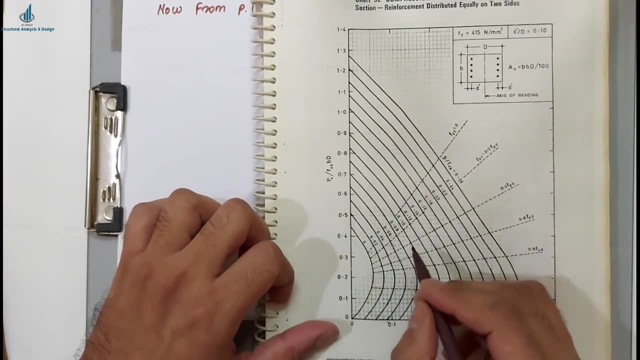 be 0.32 and the value lies in the next immediate square. so this is 0.32 and the value lies in the between this. so you have to come on this line here and from this here and you will be getting one point. so i am marked with very small dot here. so this is your point and you will be selecting. 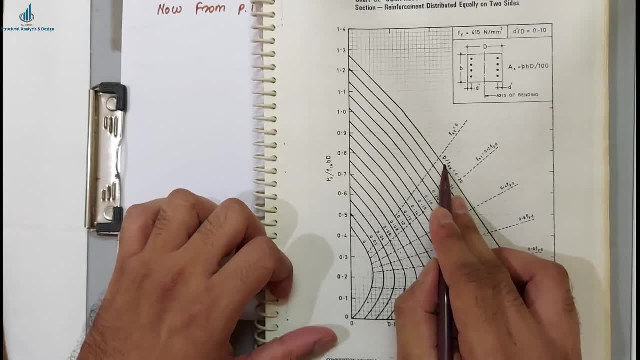 the next higher curve, which is given as p by fck. so the p by fck value for this particular calculation is 0.08. so this is first curve, second, third, fourth, so this is 0.08. so this is 0.08 so 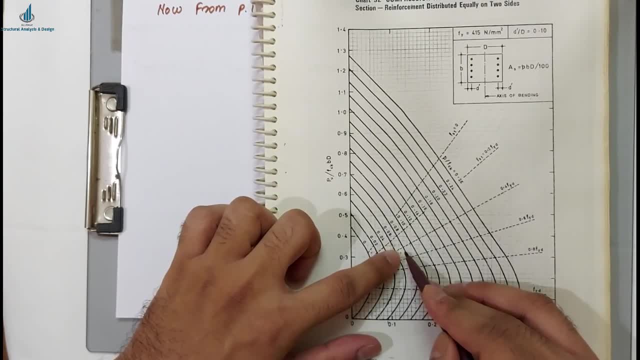 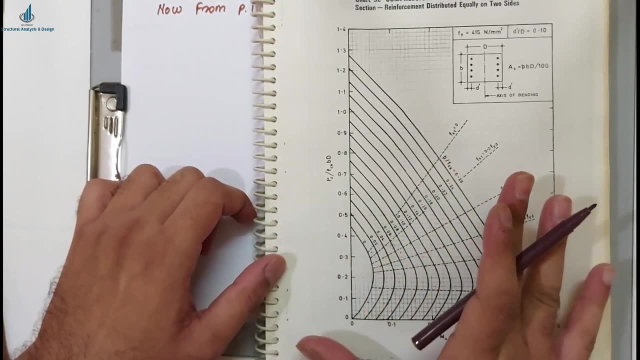 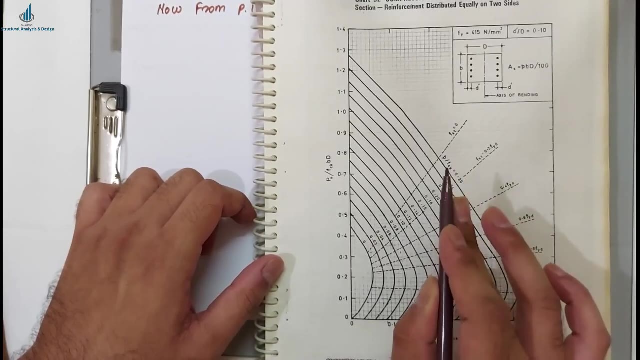 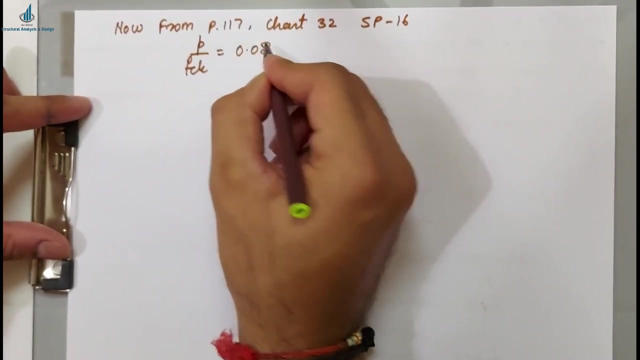 our point lies here, so we will be taking the next immediate curve. so p by fck will be 0.08. so, like this way, you have to interact with this chart and you have to get the value of p by fck and in turn you will be getting the percentage of steel p. so p by fck is equals to 0.08. therefore, 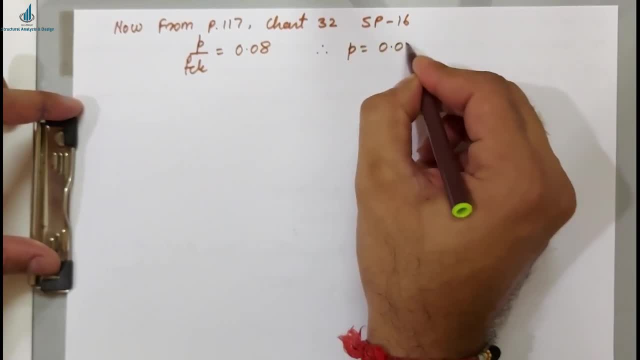 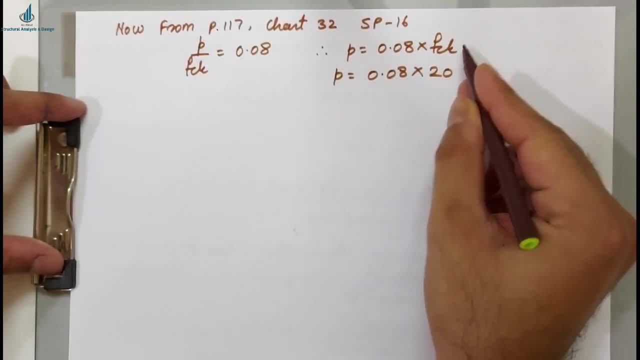 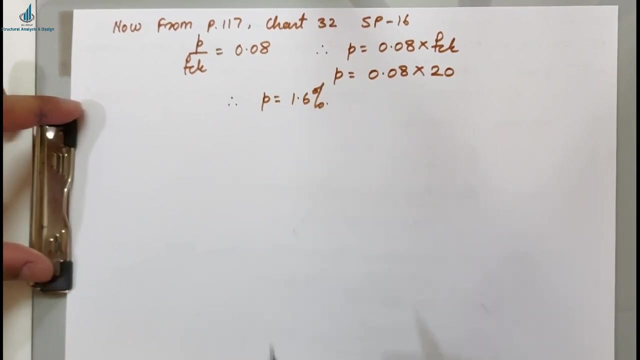 p is equals to 0.08 into fck, so p is equals to 0.08 into 20. the grade of steel was 20 newton per mm square. therefore p you will be getting 1.6 percent and it satisfies. the lower percentage is 0.8 percent for column. 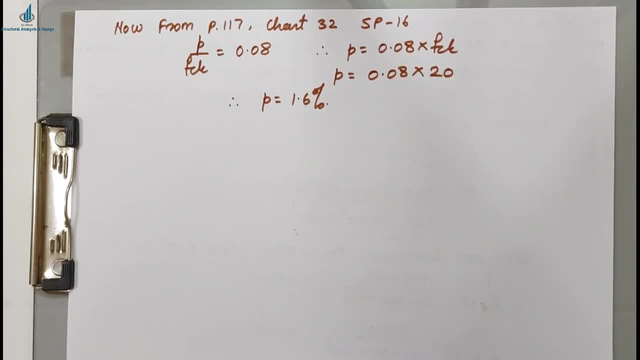 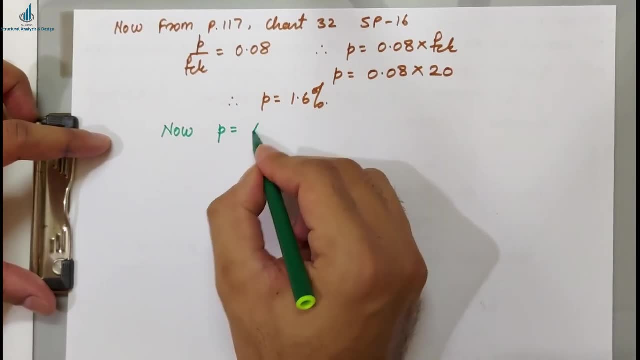 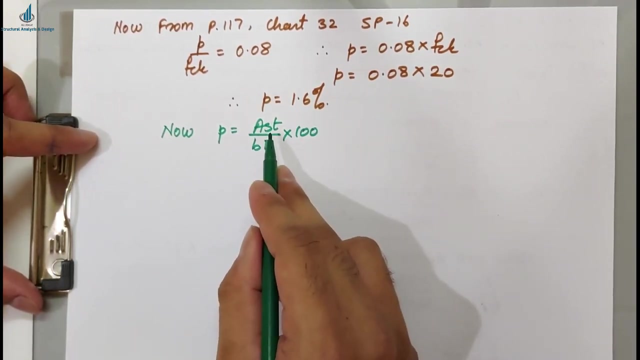 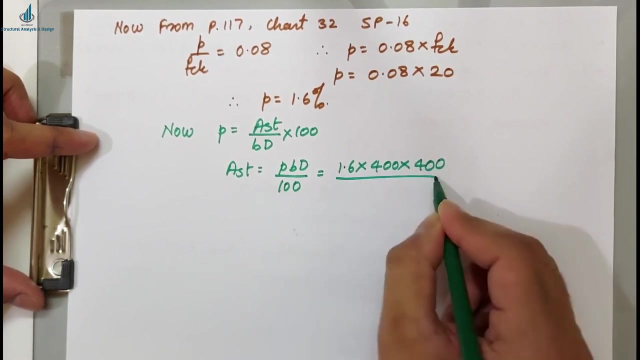 and the higher percentage is 6 percent, so it lies 1.6 percent, therefore. okay, now this p is given as ast by bd into 100. so from this now you have to find out the area of steel. so ast equals to p, bd divided by 100. so p is 1.6, b and d are 400 divided by 100, so ast will be. 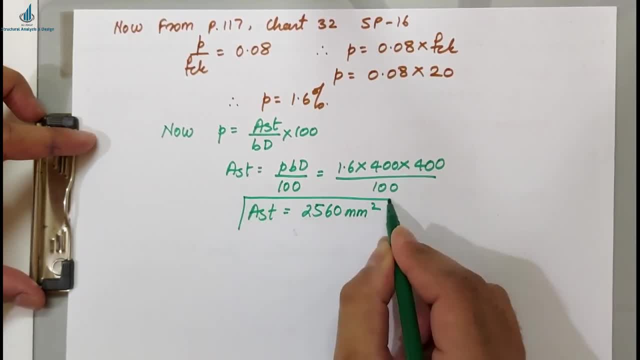 2560 mm squared, so it is 1.6. so it is 1.6 and the area of steel is 0.08, so we will be getting 1.6-1.8.. So this is your area of steel for this column and you have got this from page number 32.. 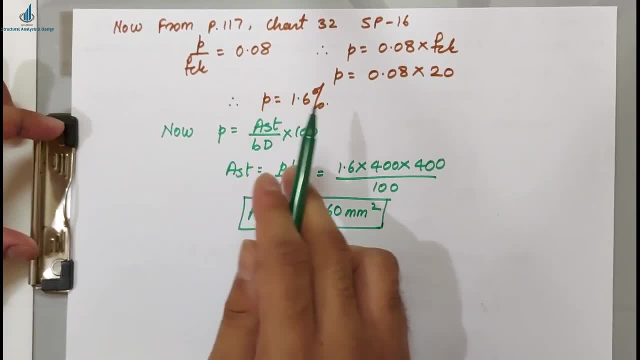 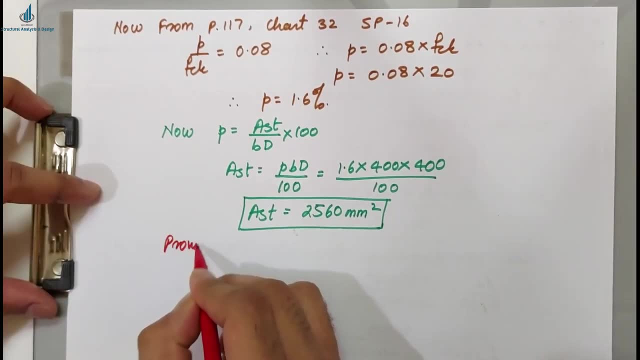 So from page number 32, the main motto is to get the percentage of steel and from that percentage of steel you will be getting your area of steel. Now provide 25 mm diameter bars, So small AST, AST of 1 bar, pi by 4, 25 square. 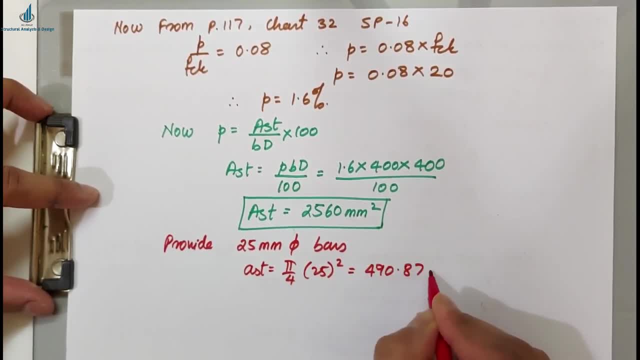 So you will be getting 490.87 mm square. Therefore, number of bars equals to capital AST by small AST. So that is 2560 divided by 490.87.. So you will be getting 5.21 bars. But 5.21 is not enough. 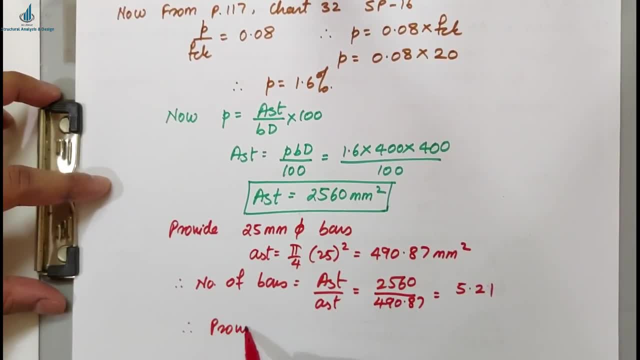 Not possible to provide. therefore provide 6 bars of 25 mm pi, 3 bars on each face. So the reinforcement was equally distributed on two sides. So 3 bars each we will provide on each face. So you have to write down this. 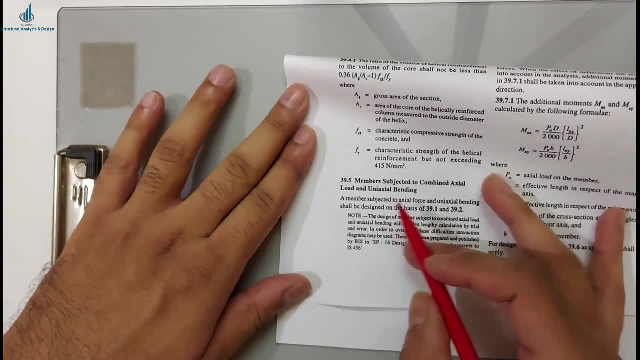 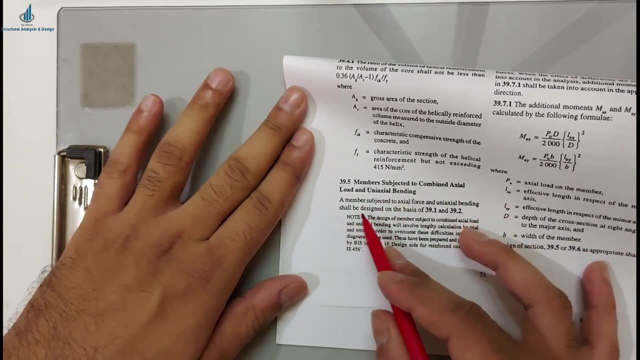 And also on page number 71 of IS-452.. Your clause 39.5 says member subjected to combined axial load with uniaxial bending. So a member shall be designed as according to 39.1 and 39.2 clause, which we have seen. 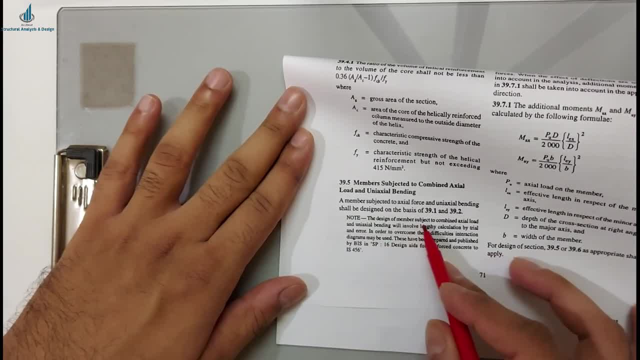 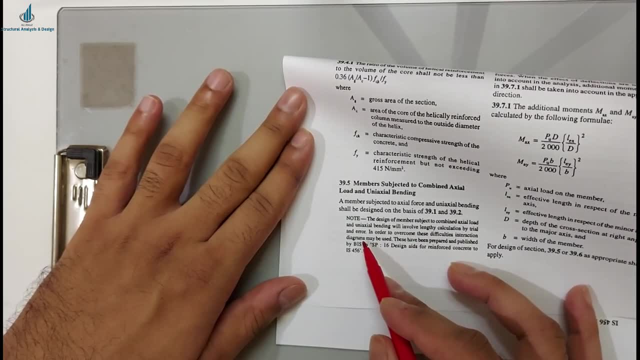 in previous videos And the note says the design of member subject to combined axial load and uniaxial bending will involve lengthy calculation by trial and error, So which I had told manually calculation. So, in order to overcome these difficulties, Interaction diagram. 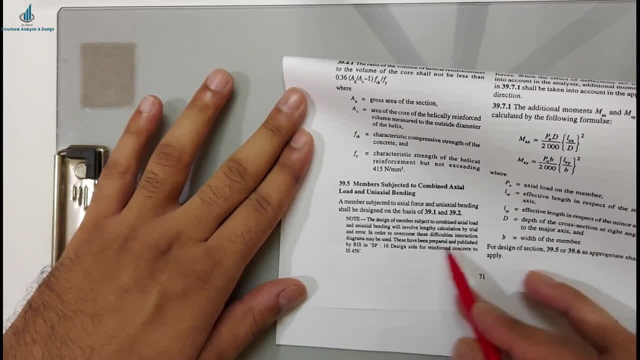 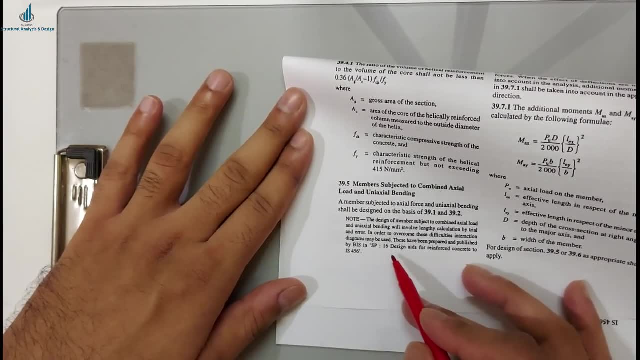 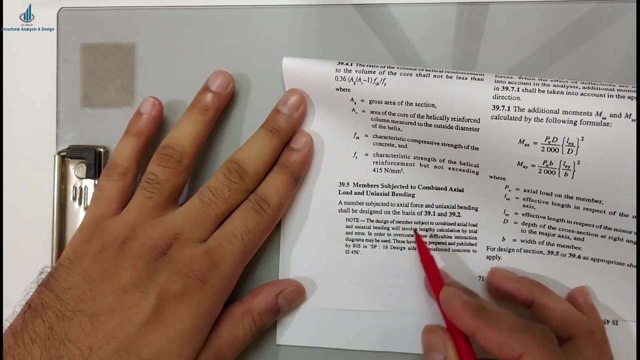 This may be used. These have been prepared and published by BIS in SP16 design aids for reinforced concrete to IS-456.. So that's why most of the practical engineers and academics follow SP16 charts. So it's very rare to go with this trial and error method, which will have lengthy calculations. 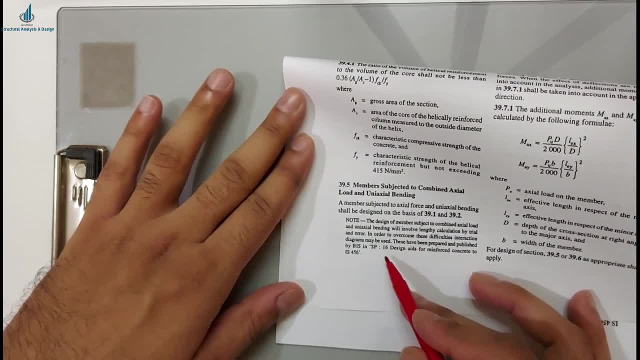 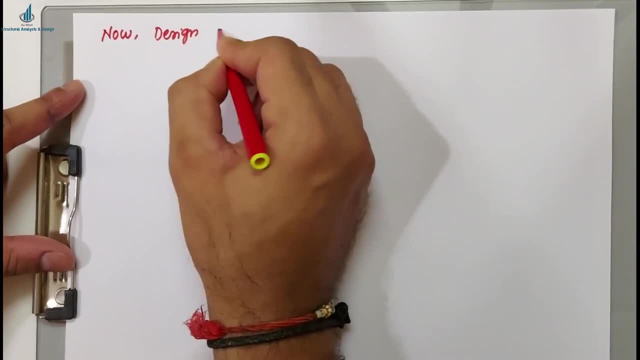 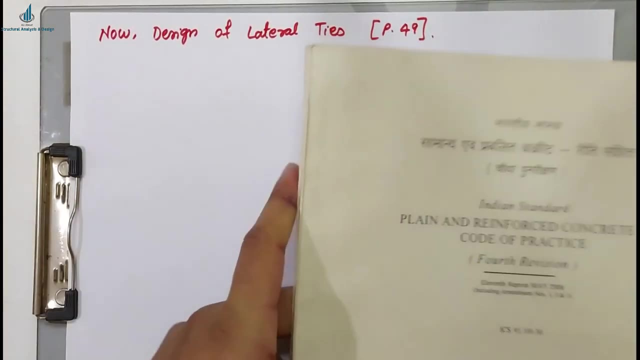 That's why. So this method we are using. So SP16 design aids for reinforced concrete. Now design of lateral. Time's this again for navigating on page number 49. So if you have seen my previous videos I have shown on page number. 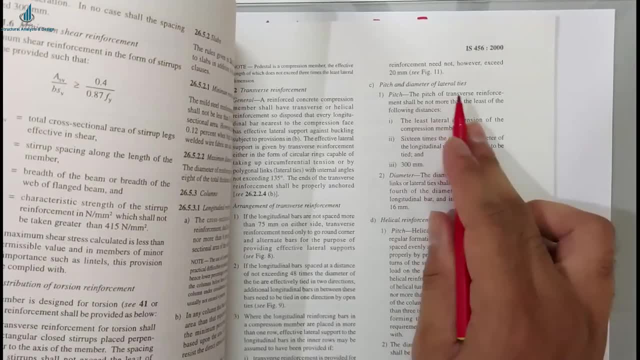 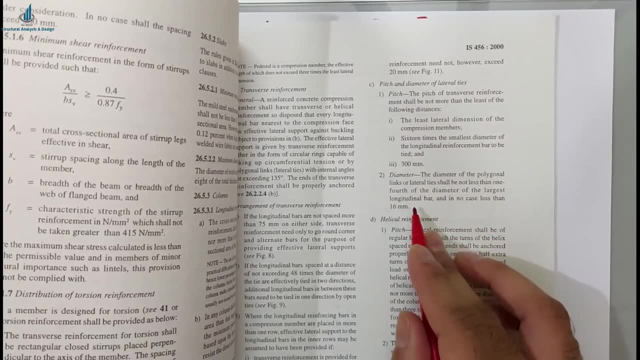 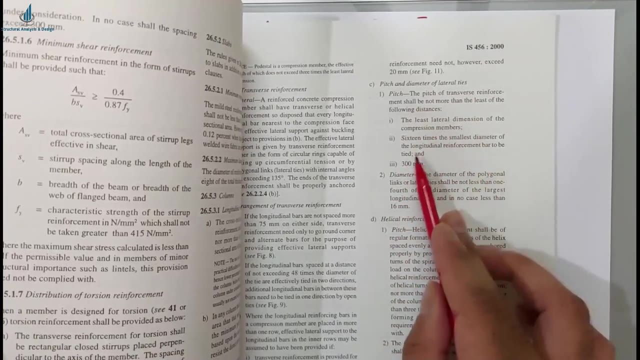 49.. So this is your page, number 49.. Pitch and diameter of lateral ties. diameter of lateral tie should not be less than 1 fourth of diameter of largest longitudinal bar and we have used 25 mm Bark Bar ties. there are again three clauses: the least you have to select, least lateral dimension 16 times. 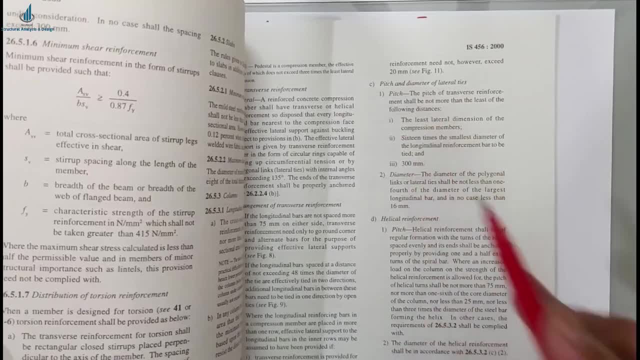 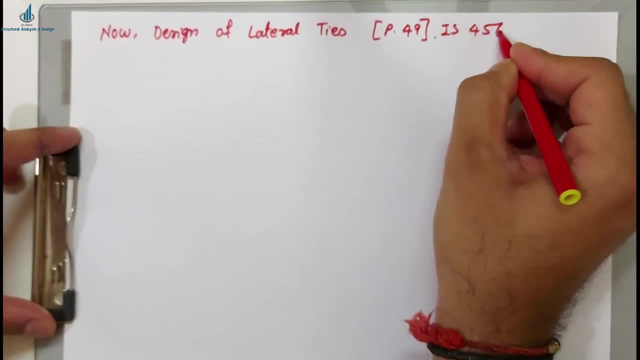 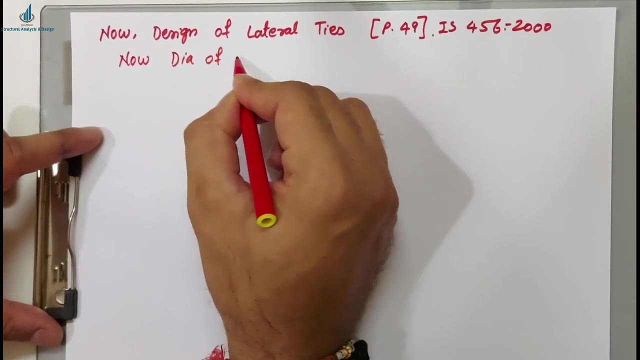 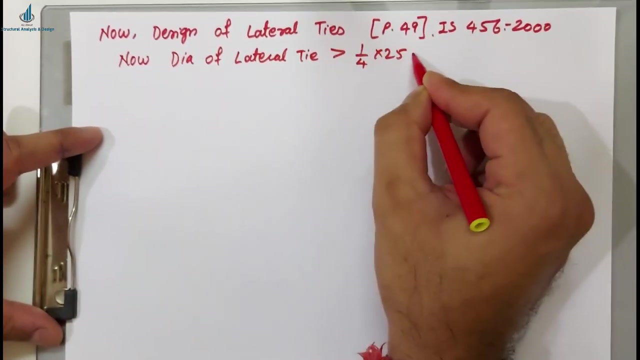 the diameter of the bar and 300 mm. so the least you have to select. so we are following this stipulation, which is given on page number 49, is 456 2000. okay, so now, diameter of lateral tie should be greater than one-fourth of 25. so this will be getting 5 point, sorry, 6.25. 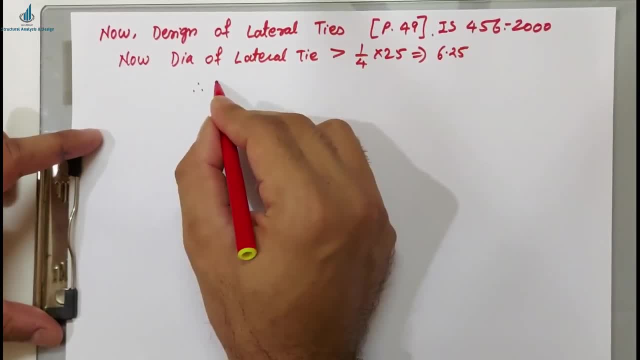 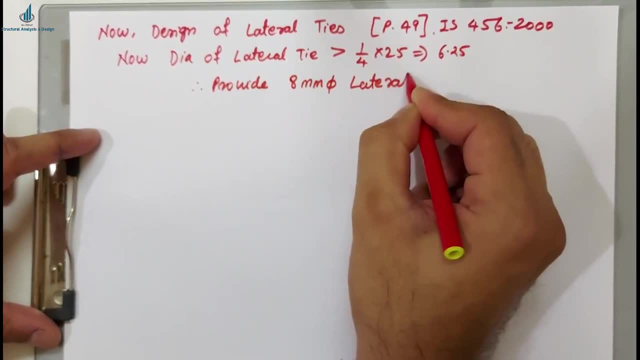 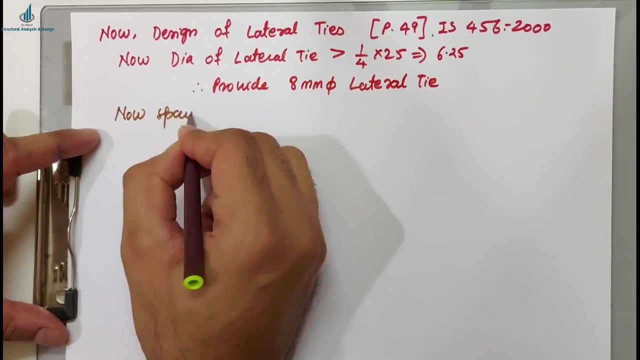 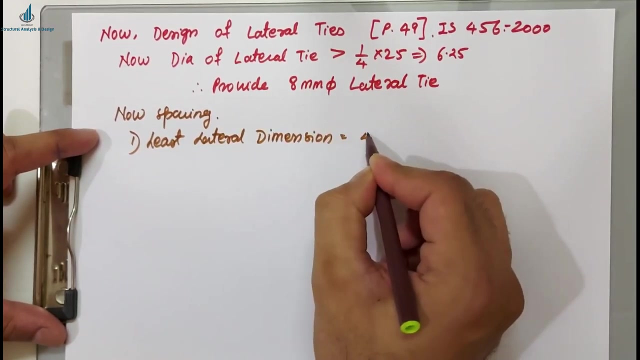 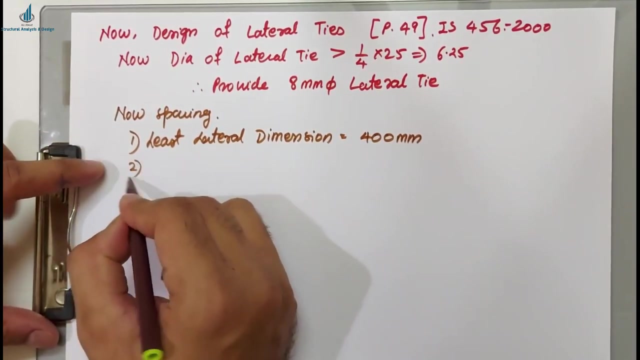 therefore provide 8 mm 5 lateral tie. okay, now spacing. so same three clauses. we have to follow: least lateral dimension, which is equals to 400 mm. the column size, 400 into 400. so if it is a tangle, the least you have to take it. next, 16 times the diameter, 16 into 25. 25 is the diameter of. 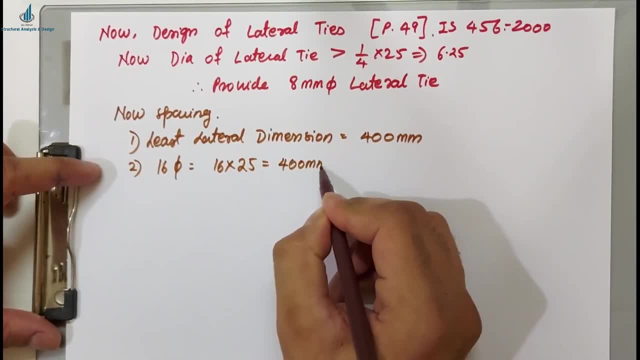 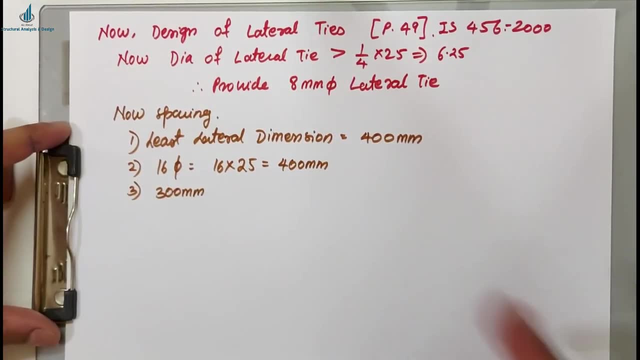 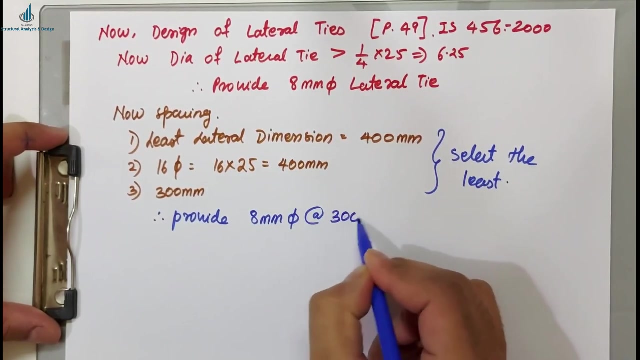 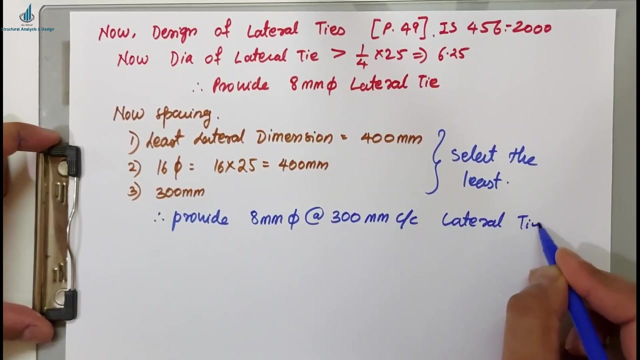 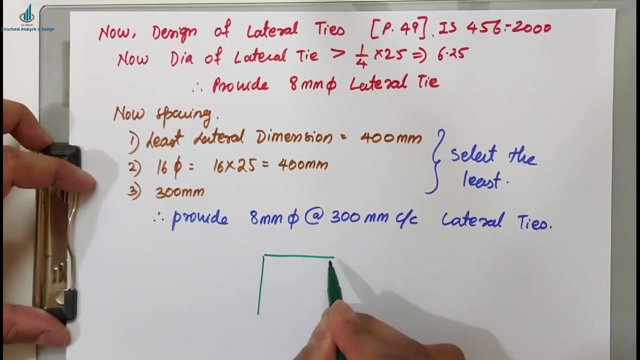 longitudinal bar. so it comes again same 400 mm. and the third clause is 300 mm. okay, so you have to select the least. therefore, provide 8mm, 5 at 300 mm. center to center lateral tense. okay, now rough arrangement, i will show you. so this is your column, so this is your 40 mm. 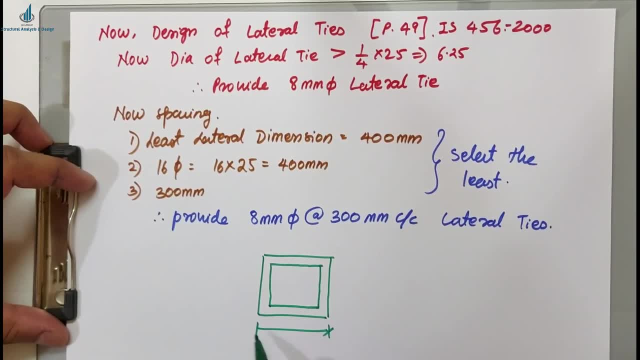 cover. so this is your 400 mm, this is your 400 mm size column, this is 40 mm D dash. okay, now in this, equally, you have to distribute the six bars, so on. here, equally we will distribute, because the chart we had referred for this kind of 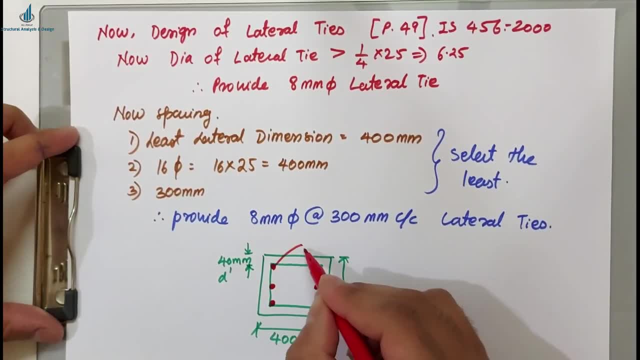 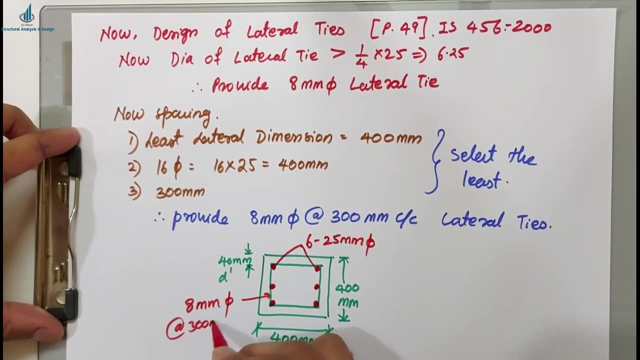 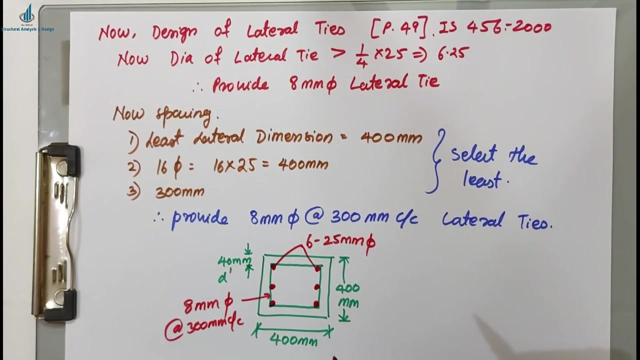 arrangement equally we have to provide. so this is your six bars of 25 mm 5 and this is 8 mm 5 at 300 mm center to center. so this is the detailed calculation of, or, or you can say, detailed design of axially loaded column with uniaxial bending of.